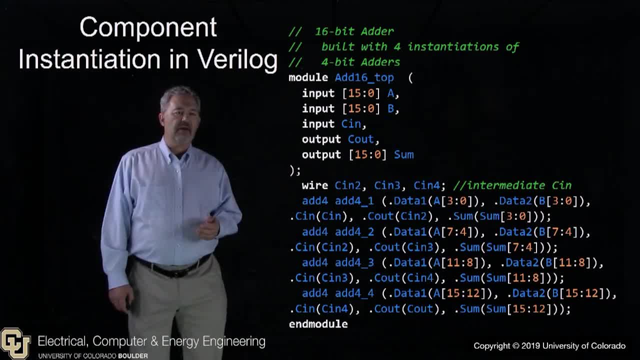 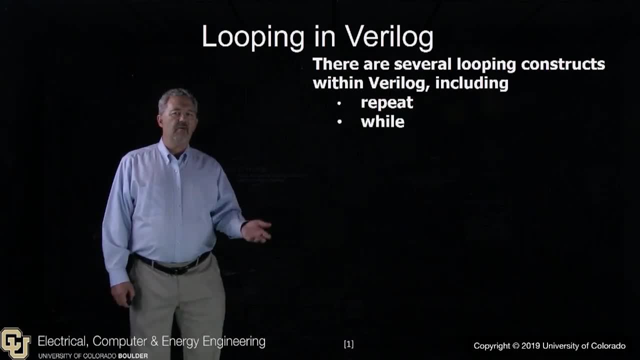 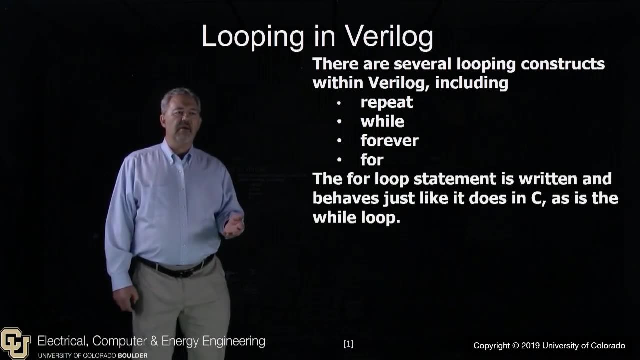 The intermediate carry wires are needed to stitch the blocks together. There are several looping construct statements within Verilog, including repeat while forever and our old friend the for loop. The for loop statement is written and behaves just like it does in C. 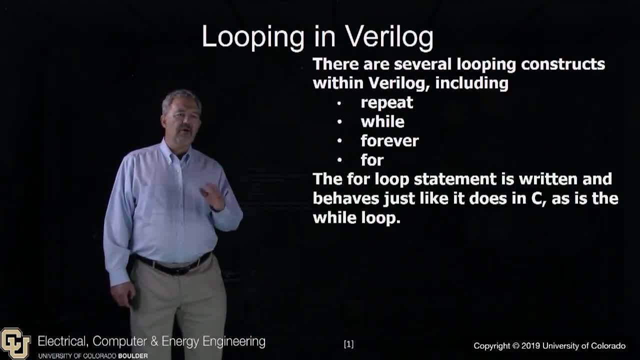 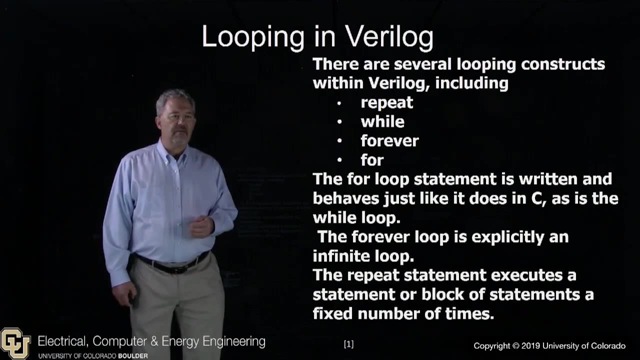 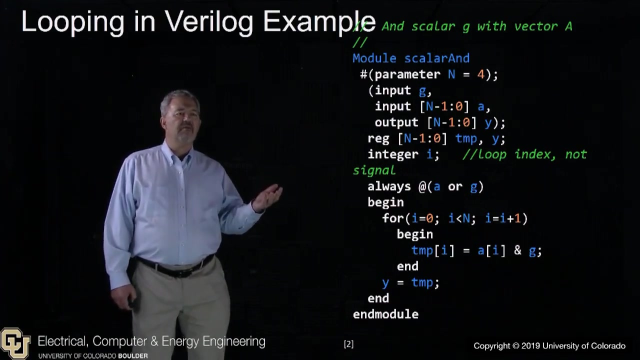 This is also true of the while loop. so if you know C, creating these loops is going to be straightforward. The forever loop is explicitly and infinitely looped. The repeat statement executes a statement or block of statements a fixed number of times. Here's a code example that uses a for loop to AND bits in a vector with a scalar signal, one bit at a time. 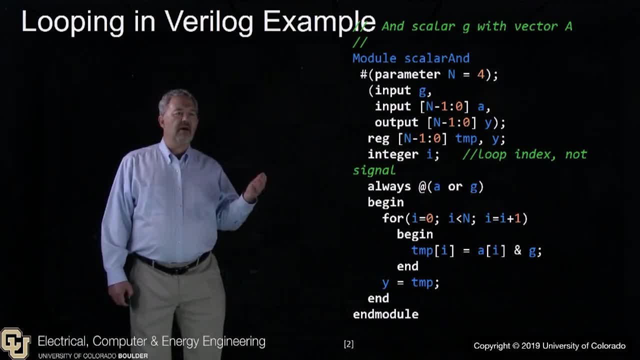 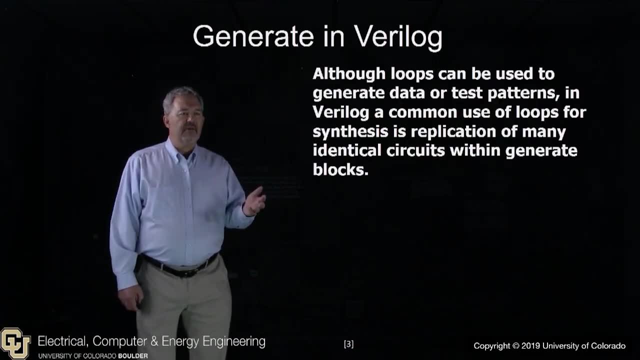 This will create N AND gates showing how the loop can create repeated copies of a circuit very efficiently. Although loops are often used to generate data or test patterns in Verilog, a common use of loops for synthesis is replication of many identical circuits within generate blocks. 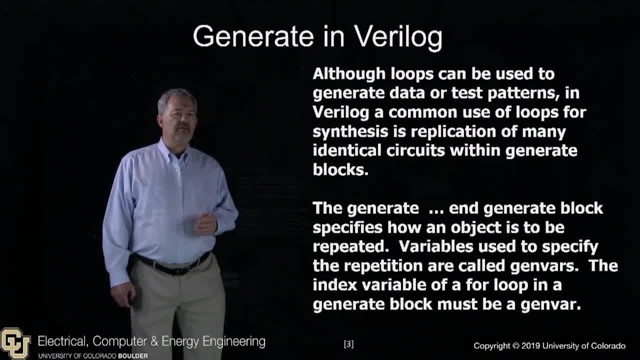 The generate to end generate block specifies how an object is to be repeated. Variables used to specify the repetition are called genvars. The index variable for a for loop in a generate block must be a genvar. Let's look at an example. In this example, we XOR two vectors one bit at a time. 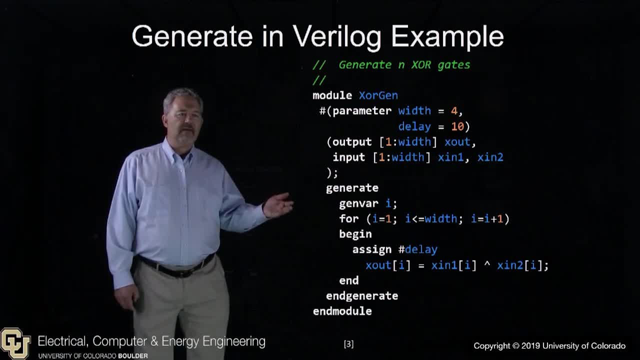 X1 gets XORed with X2, producing Xout. The delay is ignored for synthesis, but helpful for simulation. Note that this does not sequentially XOR the bits, but creates a number of XOR gates in parallel, equal to the parameter width. So in this case the for generate allows you to create many copies of a circuit. 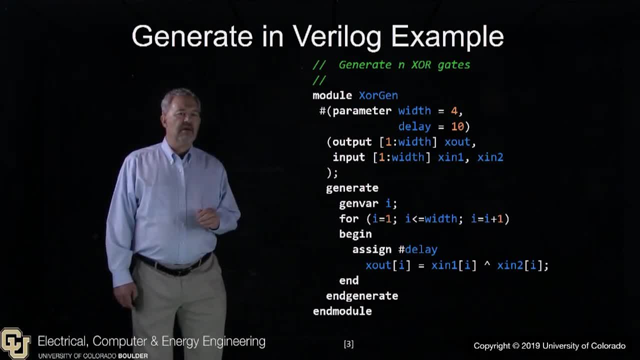 So in this case, the for generate allows you to create many copies of a circuit. Note that this does not sequentially XOR the bits, but creates a number of XOR gates in parallel equal to the parameter width. Note that this does not sequentially XOR the bits, but creates a number of XOR gates in parallel equal to the parameter width. 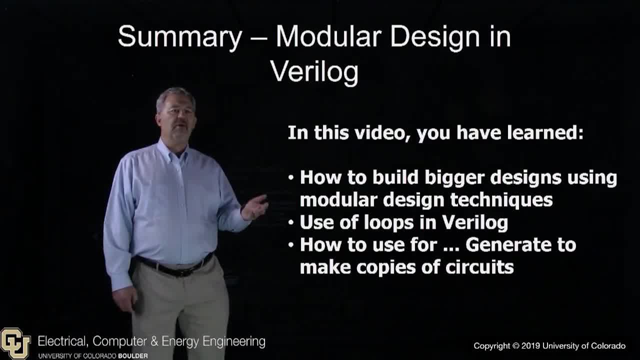 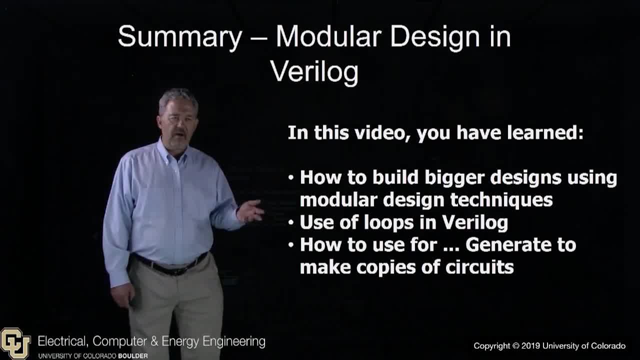 Note that this does not sequentially XOR the bits, but creates a number of XOR gates in parallel equal to the parameter width. Note that this does not sequentially XOR the bits, but creates a number of XOR gates in parallel equal to the parameter width. Note that this does not sequentially XOR gates in parallel equal to the parameter width. Note that this does not sequentially XOR gates in parallel. equal to the parameter width.